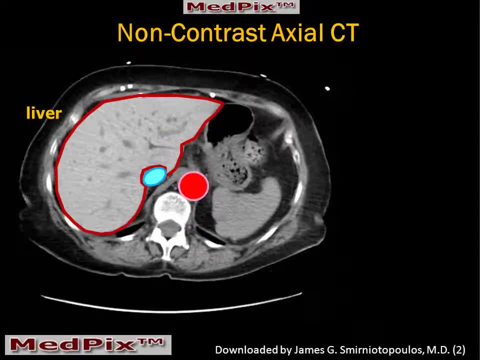 We can see the abdominal aorta, the inferior vena cava. we can see the liver, the stomach with some food contents and we can see the spleen. Normally the liver is slightly hyperdense or hyperattenuating or wider than the muscles. 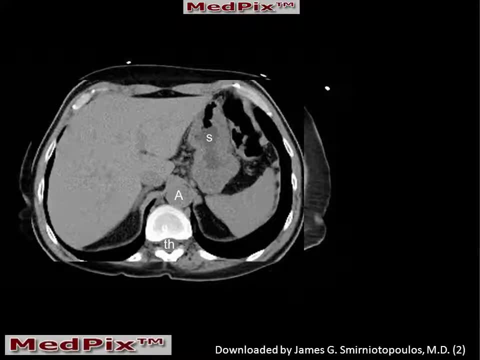 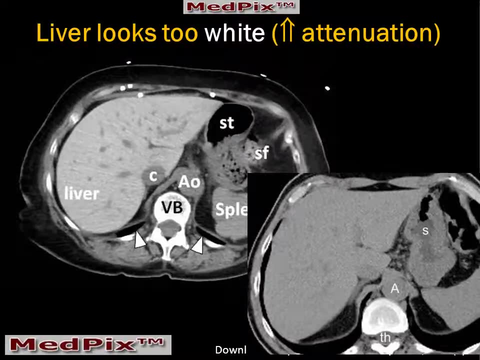 and the spleen on a non-contrast CT scan. But if we compare this patient's scan to our patient, we can see that in our patient the liver looks way too white. The attenuation seems to be way too high. How can we confirm this? 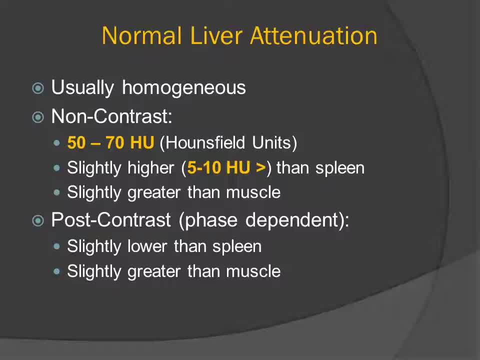 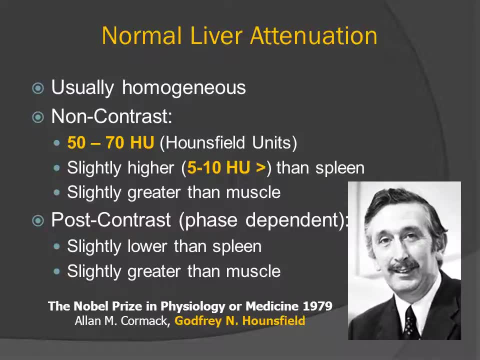 The normal liver has 50 to 70 Hounsfield units, and it's typically 5 to 10 units higher than the attenuation of the spleen. Of course, these Hounsfield units are named after Godfrey Hounsfield or Sir Godfrey Hounsfield, who won the Nobel Prize in Physiology or Medicine in 1979. 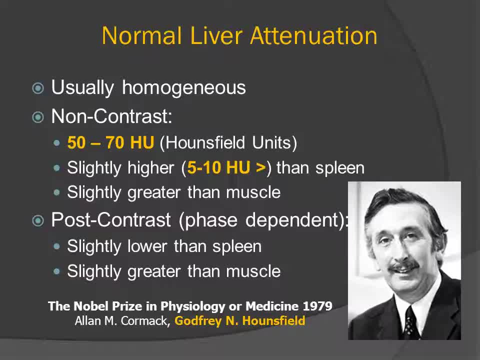 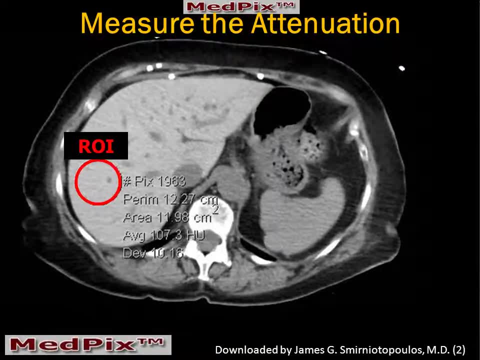 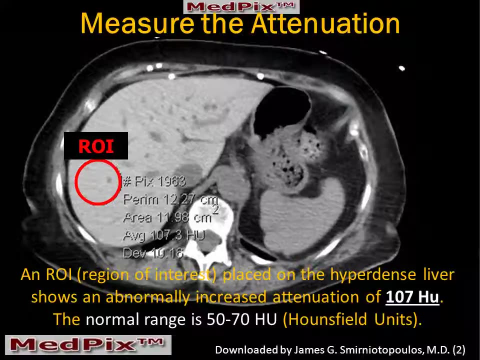 for his invention of the CT scanner, along with Alan Cormack. If we actually measure the attenuation of the liver using an ROI or region of interest in our patient, it's 107 Hounsfield units and the normal range is only up to 70 Hounsfield units. 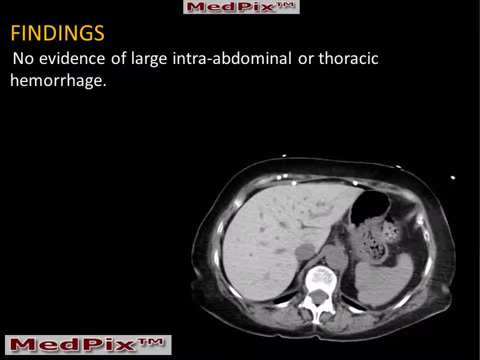 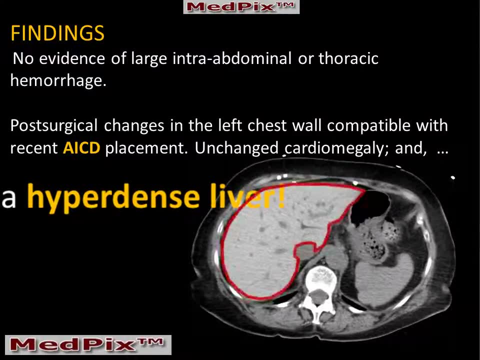 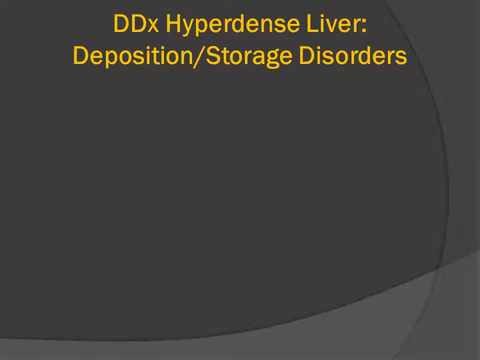 So this patient's liver is way too high in attenuation. So this patient's liver is way too high in attenuation. We also see some post-surgical changes, but the hyperdense liver is the main finding in this particular patient. So what is the differential diagnosis for a hyperdense or hyperattenuating liver? 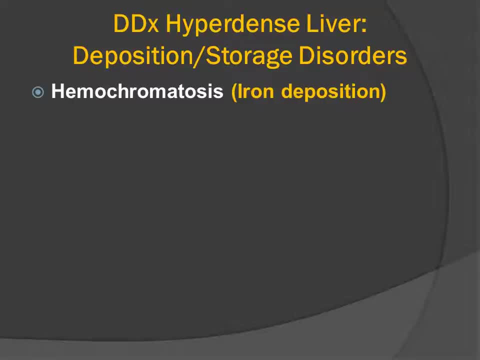 Most commonly, it's going to be due to a deposition or storage disorder. Hemochromatosis where iron is deposited may be hereditary or may be secondary to a number of processes, including blood transfusions, increased oral intake or ineffective erythropoiesis, such as occurs in thalassemia. 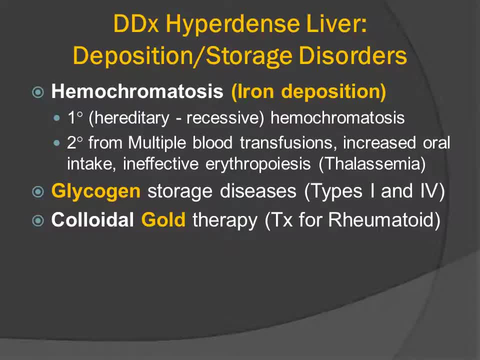 Glycogen storage disease. colloidal gold therapy, which has been used for rheumatoid arthritis. Wilson's disease, where copper is deposited in the liver. Thoratrast, which was a contrast medium used in the 1920s to 1950s and contained thorium. 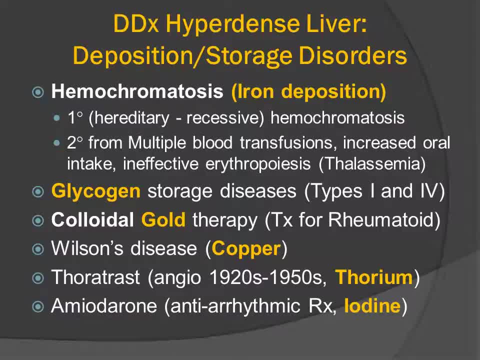 And amiodarone, which is an antiarrhythmic drug that contains iodine. Amiodarone is an antiarrhythmic drug that contains iodine. Amiodarone is an antiarrhythmic drug that contains iodine.